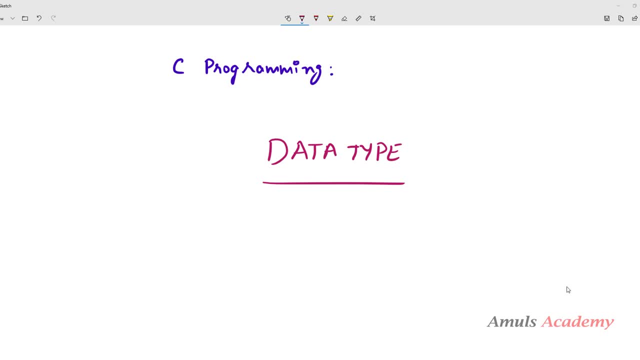 Hello guys and welcome to C programming tutorials by Amuls Academy. We were discussing about data type. Next we will discuss about data type modifiers in C programming language. Modifiers are the keywords in C language, which changes the meaning of basic data type. So these modifiers. 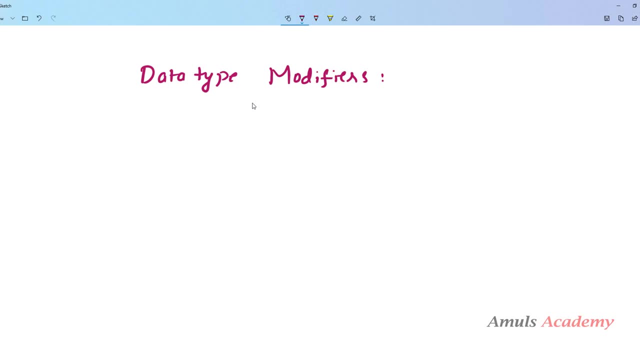 are used as a prefix to the data type to redefine the size and range of the data type. So the syntax is: first we need to mention the modifiers, Next, data type: the basic data type, like int, char. Next, here we need to mention the variable name. Ok, so this is the 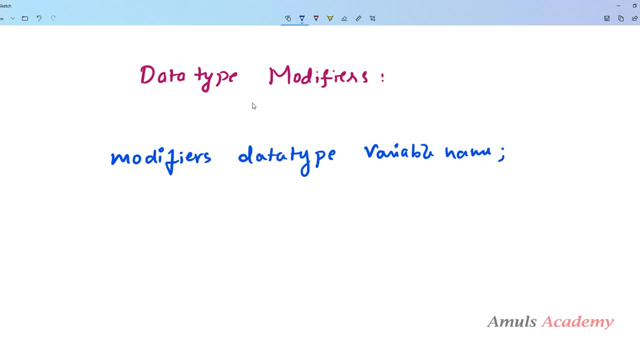 syntax Modifiers are used as a prefix to the data type. Next we will see the different types of modifiers. There are actually five modifiers in C programming language, So we will see short, long and long, long, signed unsigned. So this short, long and long, long. 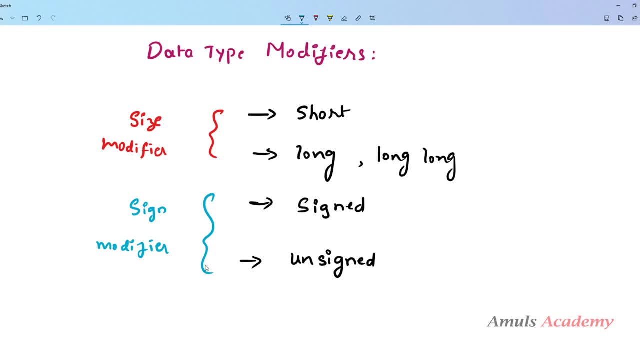 are called as size modifiers. Signed and unsigned are called as sign modifiers. Let's discuss each modifiers in detail. First we will discuss about short modifier. We can use short modifiers only with the int data type. As I explained earlier, int data type take different memory space, like 2 byte, 4 byte or 8 byte. It depends. on the computer architecture and compiler right. If you want to allocate the fixed memory space for the int, then you can use this short modifier. So the size of the short modifier is 2 byte. So if you want to store small integer value then you can use this modifier with. 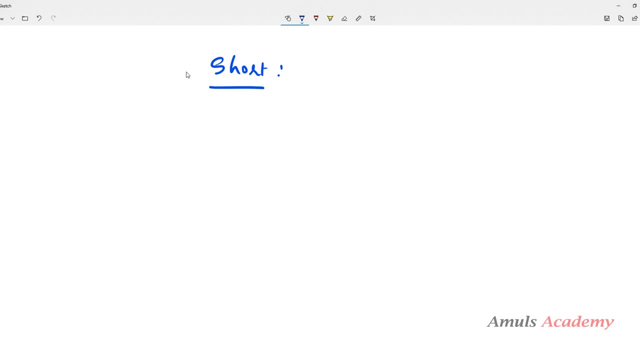 the int data type. It takes less memory. So for that we need to take short key word first, Next, followed by the int data type. Next you can take any variable name, like a. So if we didn't mention the data type, for example, if you just mention short, 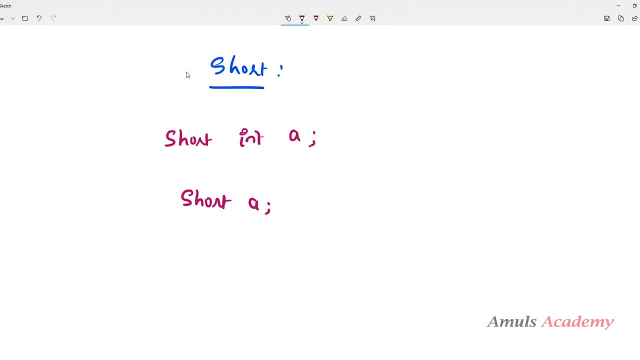 a. then also it will take the default data type as int, because we can use this short modifier only with the int data type. So you can mention like this also. So size of short modifier is 2 byte, So range will be from 2 byte to 12 bytes. So you need to take the 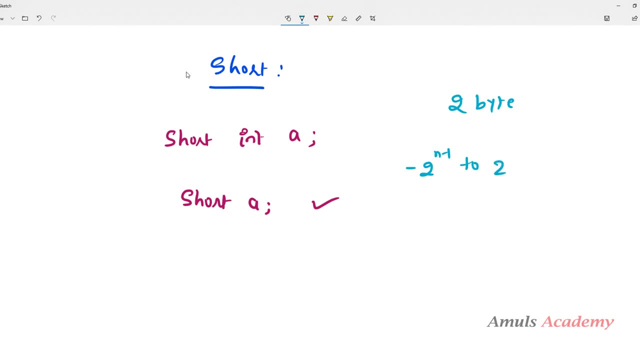 be from 2 power n-1 to 2 power n-1-1. so n is nothing but how many bits it will take to store in memory. so 2 byte is nothing but 16 bits. so here: 2 power 2, 2 power 15-1. ok. 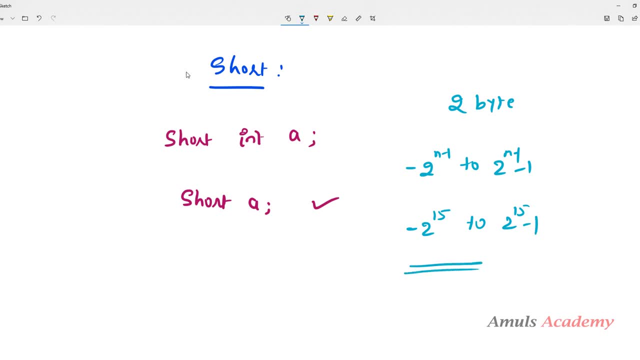 so this is the range. all right, so this is about the short modifier. next we'll talk about the long and long, long modifier. so you can use these two modifiers when you want to increase the size of the current data type. we can use this long data type with int and. 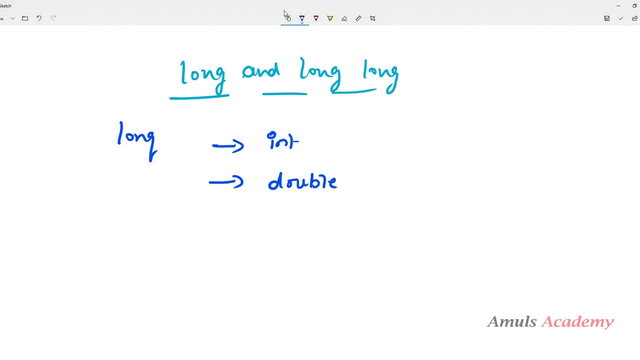 double. we can't use this with the character or float. the size of this long modifier is 4 byte or 8 byte. it depends on the computer architecture and compiler syntax is we need to take long int a for the double. you can take long double b like this, so if 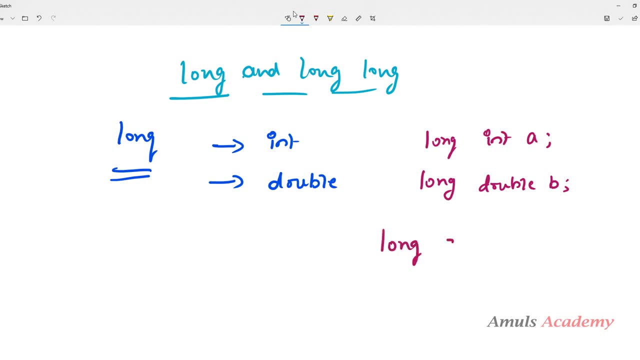 you didn't mention the data type. for example, if you just mention long c, it will take the default data type as int. ok, it will treat this as long int c. ok, so the default data type for the long is integer. all right. Next about the long, long. 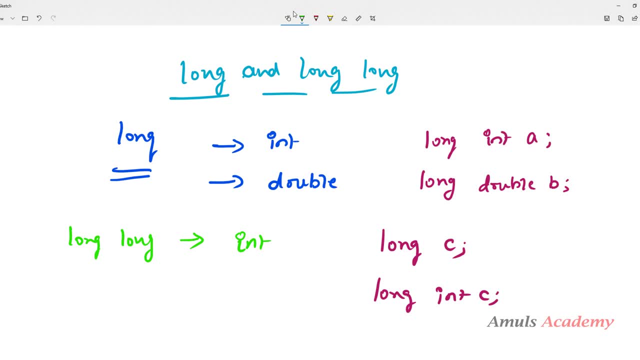 We can use long long with only integer, so the size of long long is 8 byte and the example is: you need to mention long, long int a like this: ok, or you can just mention long long a, ok, so this is about the short, long and long long modifier. 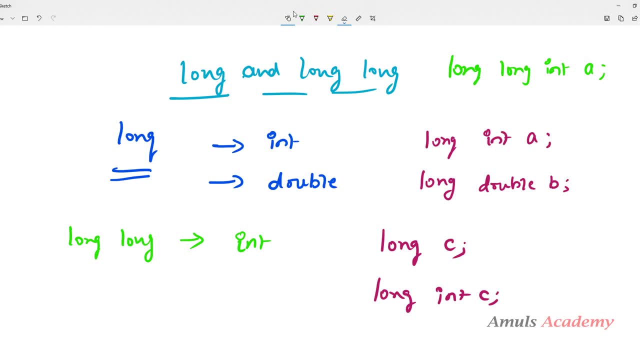 Next we'll talk about the signed modifiers, that is, signed and unsigned modifier. so first we'll talk about the unsigned modifier. we can use this unsigned keyword with the int and character data type. this keyword can be used for those variable which can take only values which are 0 and positive. it won't take the negative values, ok, and the example is: 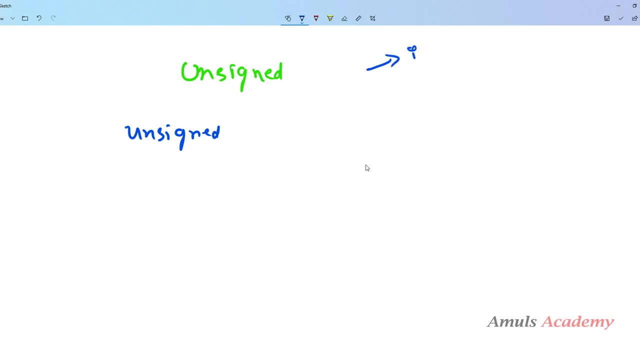 unsigned. we can use this with int and character. all right, so unsigned, int a. so that type. this variable only takes negative values. ok, and the example is unsigned. we can use this with it. take the positive value and 0, it won't take the negative value. 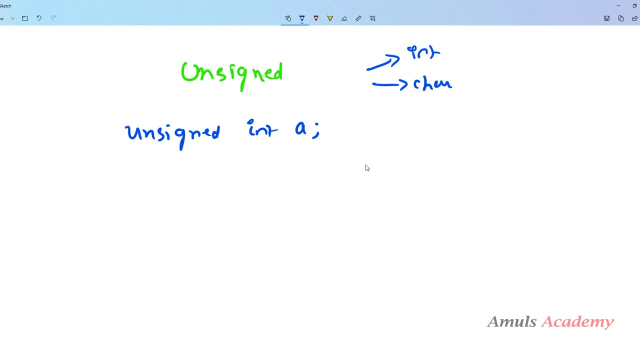 So that's why if i take unsigned int a, then the range will be from 0 to 2 power n minus 1. so 0 to 2 power n is nothing. but if the size of int is 2 byte, ok, so 16 bits right. 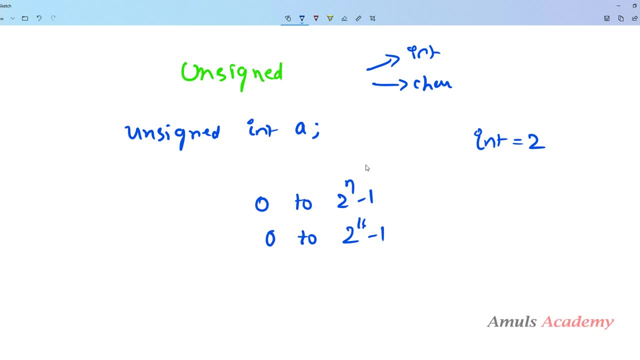 2 power 16 minus 1. this will be the range for the char unsigned character. b character will take 1 byte right. So the range of this will be 0 to 2 power n. 2 power n is nothing but 2 power 8, because 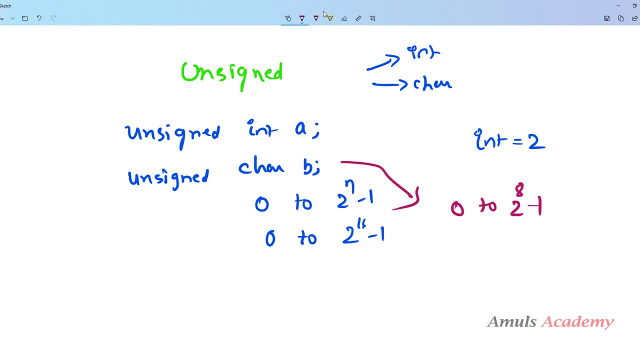 character. take 1 byte. 1 byte is nothing but 8 bits minus 1, so this will be the range 0 to 255. so it only takes positive values. and if we didn't mention any data type, with the unsigned modifier, by default it will take int as the default data type. for example, if 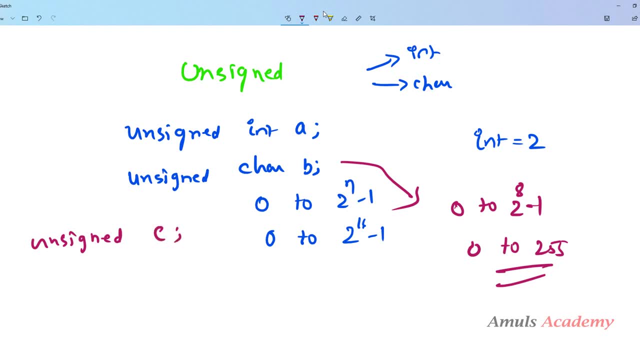 i take unsigned int, i will take int as the default data type. for example, if i take unsigned c, so it will take default data type as int. So this is about the unsigned modifier. next we will talk about signed modifier. so we can use this signed modifier with the int and char. it is the default modifier for the int. 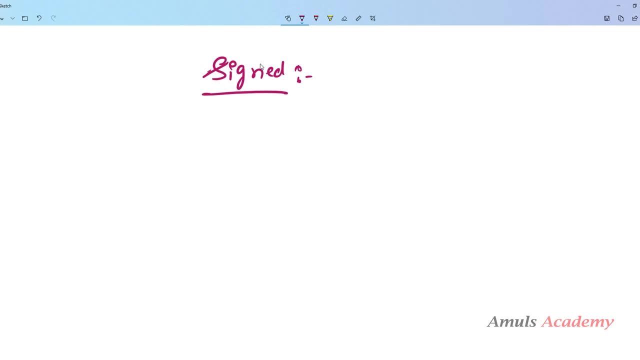 and character data type. if modifier is not specified. for example, if i just mentioned Int a, so it will take both positive and negative value, right? so the default modifier here is signed. so this signed modifier allows the variable to store negative value, positive value as well as 0. if i take int as 2 byte, so range will be from minus 2 power n minus. 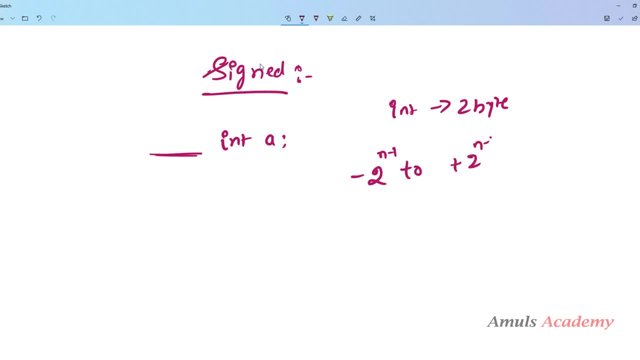 1 to plus 2. power n minus 1 minus 1. that is nothing but minus 2. power 15 to plus 2. power 15 minus 1. so this will be the range. if you are mentioning signed modifier, then you need to mention signed int a, like this, signed character b, something like this in the case: 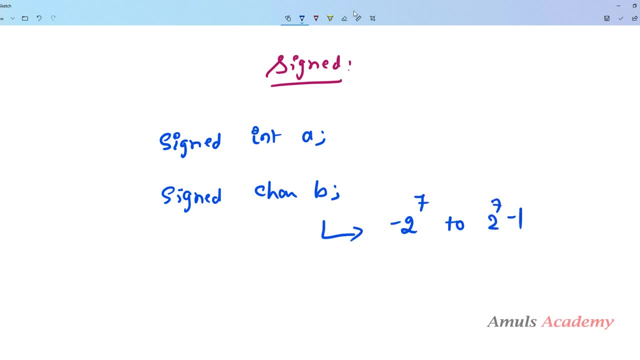 of character range will be 2 power 7 minus 1, that is, i guess, 128 to 127. this is the range for the signed character. so for the unsigned modifier the formula is 0 to 2 power n minus 1. for the signed modifier, formula is minus 2. power n minus 1. to plus 2. power n minus.